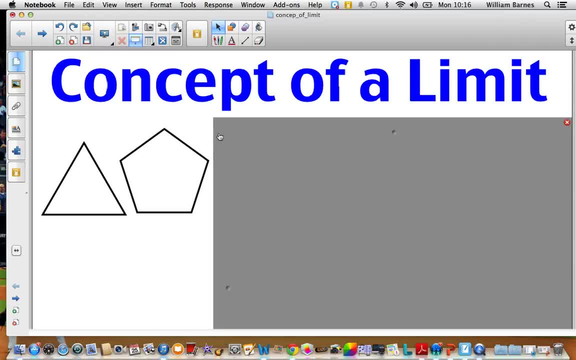 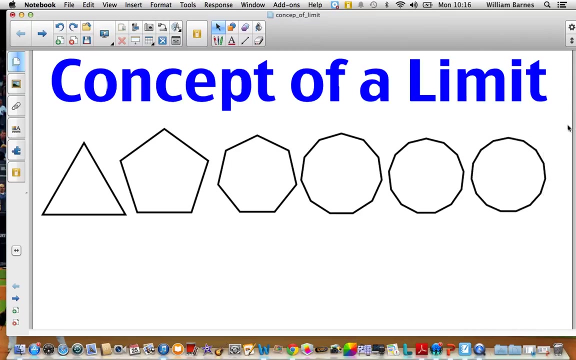 Still not really close to a circle. So then we go to seven sides. You know it's getting a little bit closer to a circle. Then let's go to nine, You know, a little bit closer still. Then we have 11, and still a bit closer, and then we go to 13.. So you can imagine what would happen if I kept adding sides and sides and sides and sides. 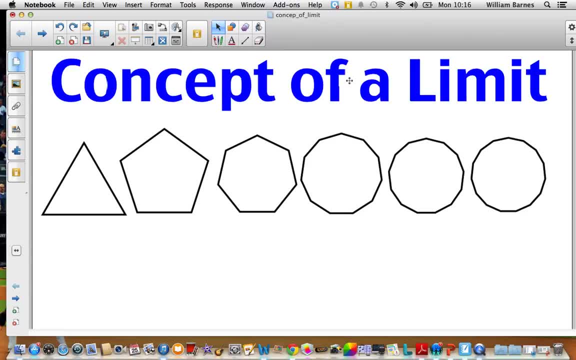 You know, eventually I would get a pentagon. Eventually it keeps getting closer and closer and closer and closer to looking like a circle. But is it actually a circle? Well, no, because if we zoomed up on it we would have, you know, little sides if we got really, really close to it, So it wouldn't actually be a circle. 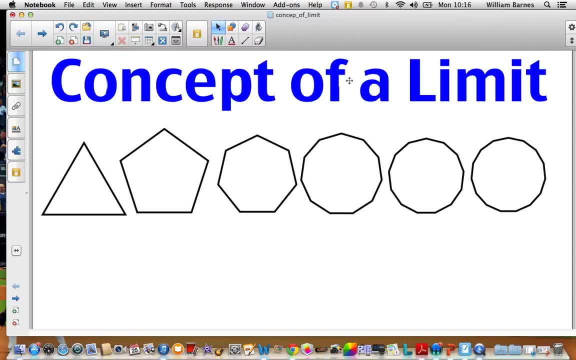 The only time it would actually be a circle is if we can somehow go to infinity and get as close to a circle as possible. That would be an infinite number of dots or sides. So you know, the idea of a limit is that you're approaching something And you know, in this case, the limit was the circle. 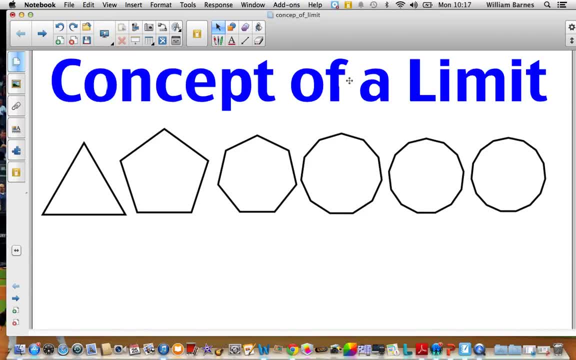 You know, as we add sides, we're approaching, we're getting closer and closer to this idea- the shape of a circle. Well, with numerical limits, we're getting closer and closer and closer to a number. So this is what you might see. you know, in your first couple days of calculus class, You might see a graph like this: 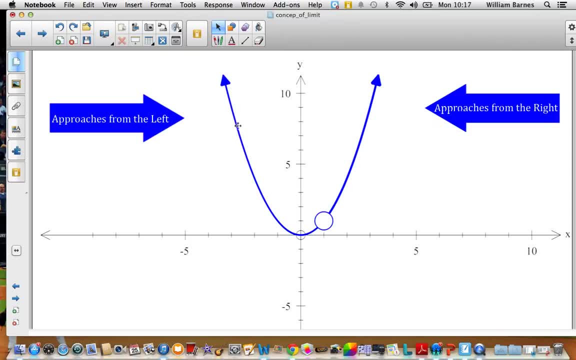 And your prof comes in and tells you: well, as you approach from the left side of your graph and you're, you know you're going down it. Maybe I'll get a marker out here, Let's get rid. And you're going down it from the left side, You're going this way. 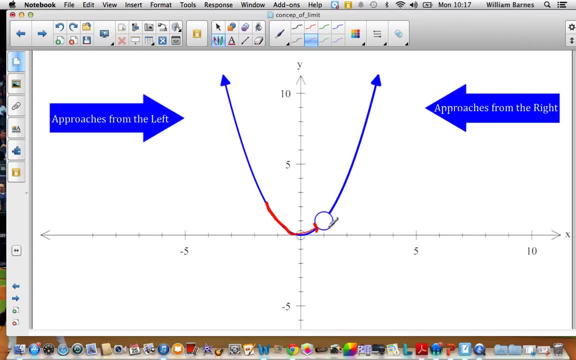 You're getting closer as we approach this empty circle. We're not really sure what's happening there. As we approach it, we're getting closer and closer to well, we're getting closer to one right here, this guy, And then we do the same thing from the right side. 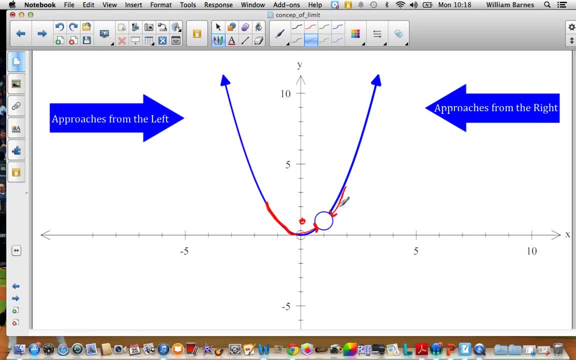 You're right. We're going down this red, this graph, And as we approach from the right side, we're approaching again, we're approaching one. So how you might write that and this is what it looks numeric in. you know what you'll the form, you'll see the limit. 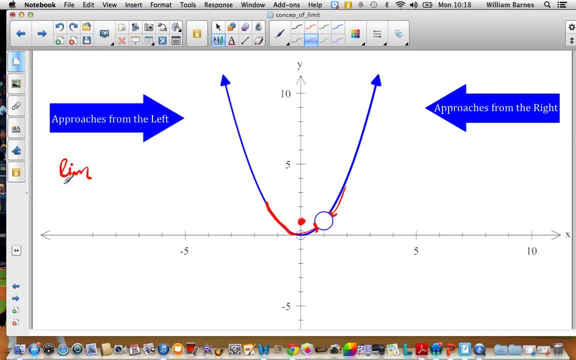 I'm actually going to try to write really neat Now. I usually hand write my limits. It's really hard to do when you're doing like with a pen tablet. As X approaches one From the left side, So X approaches this one. 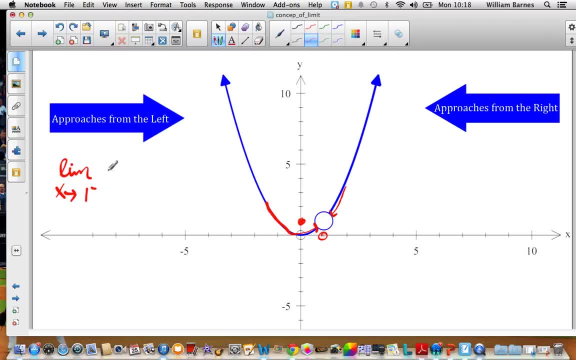 Maybe I should have picked a different graph, But anyway, of F, of X, so whatever the function might be is actually equal to this one. So while Y is essentially one, And then from the right side limit as X approaches, one from the right side. 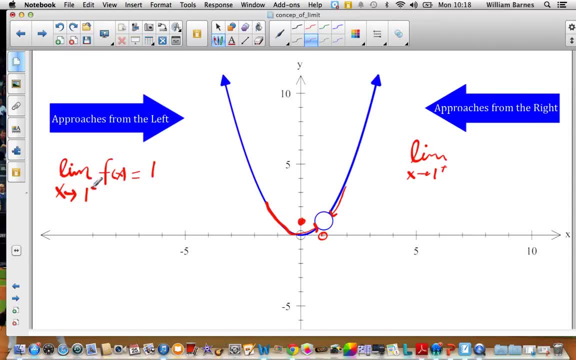 So you notice that I use a little negative- sort of a negative- as the exponent, or whatever you want to call it, A superscript. And then the same thing for this plus sign. The minus sign mean from the left, The plus sign mean from the right. 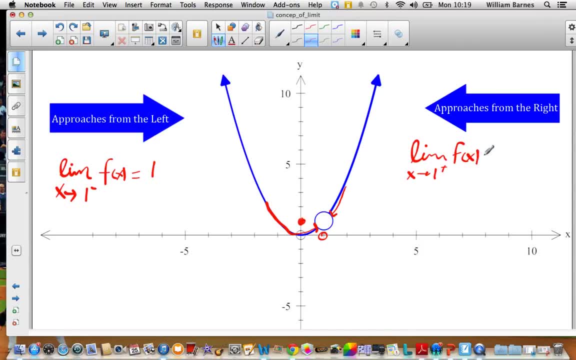 Of F of X Is equal to one. So what we notice is that as we approach from both sides, we're approaching the same number. So that's another fundamental concept of the limit: That in order for a limit to exist, it has to approach the same number from both sides of the graph. 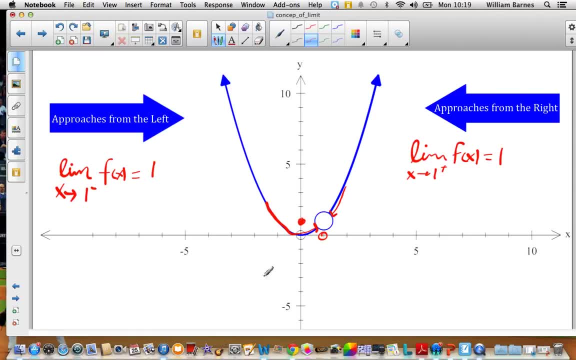 So if I have this, What I can say from this, Based on having these two things, I can then make the conjecture. If only if these things are true, I can say this: I need to have both of these things truly equal the same number. 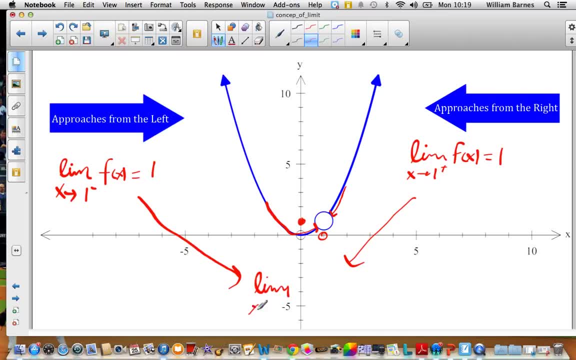 Then I can say: the limit As X approaches, one Of F of X Is equal to one. So all I'm really saying with this Is that as it gets really, really close to one here, Really really close to it. 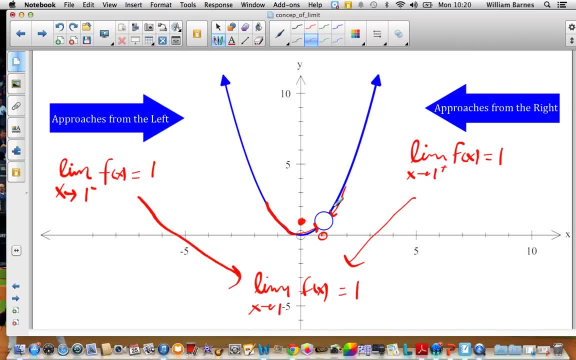 The graph is on the fine, actually at one, So we can't actually get to one, But as it gets really, really, really, really, really close to it, The value of my graph Y, F of X is also one. 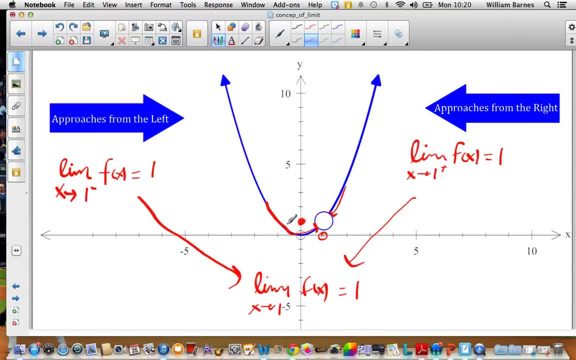 So It seems like the idea of a limit seems like such a complex topic, But it's actually fairly straight forward When you break it down. So let's have a look at another graph And see what you guys think of it. So let's. 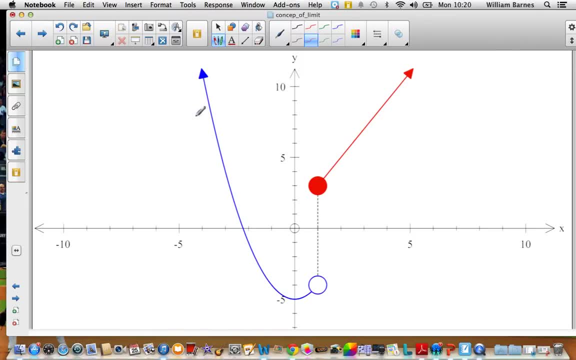 Do the one side limits for this guy. So if I look at, This is from the left side. So the limit As X approaches And we're going to go with Let's see One, two, three, four. So that's one again. 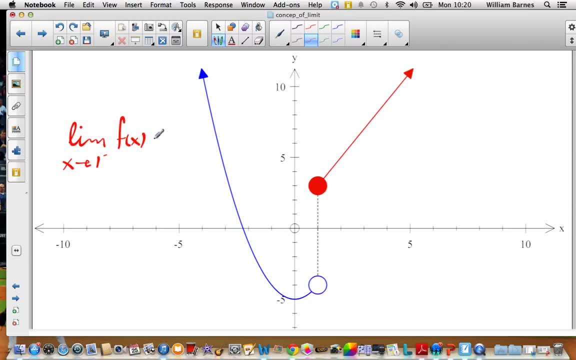 X approaches one from the left side Of F, of X- And this is a piecewise graph And these are very common in first year calculus- And it approaches, If you look here, Four. So we go across from that point Right there at negative four. 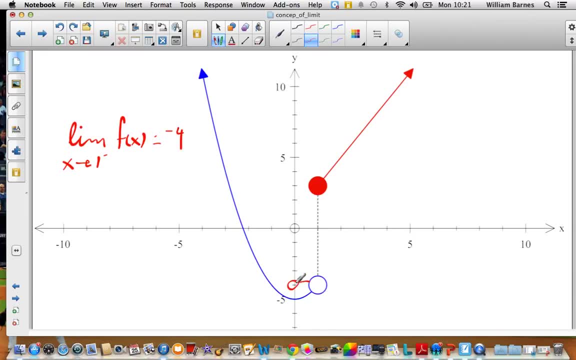 So as You approach here to one, It goes to negative four Now from the right side. Limit The lin. Let's see. Try that again: The limit As X approaches one From the right side. So you're. 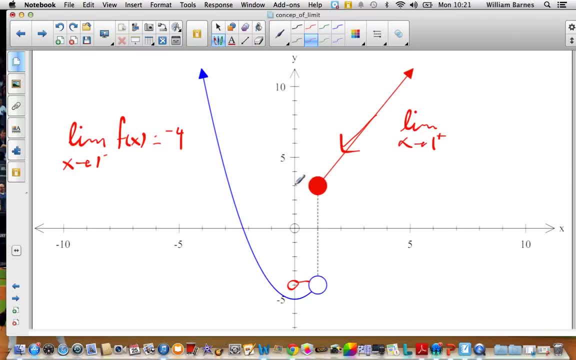 Getting really, really close to here. It looks like we're approaching One, two, three. So Of F, of X Is equal to three. So if you look at it, Our one side of limits are not equal. So what we? 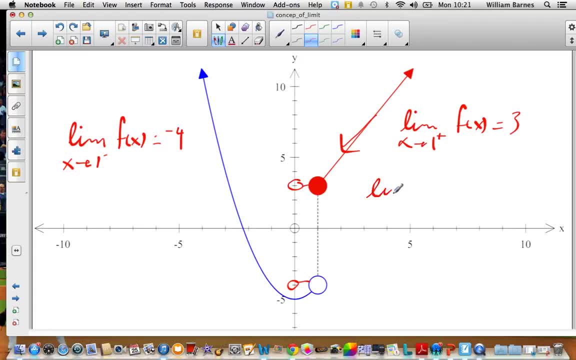 We can't really say anything about this. All we can say Is that the limit Of X approaches one Does Not Exist. That mean girl moment, right, The limit does not exist. So Yeah, that's really That's. you know, that is. 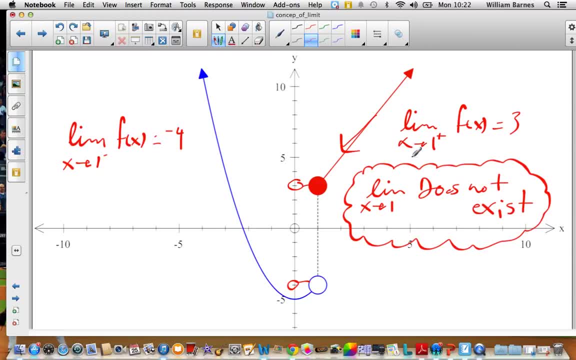 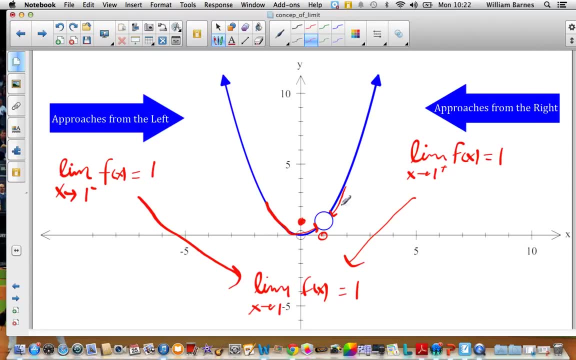 Fundamental to understanding of limits Is that limits have to approach the same From both sides. So both one side limits have to be the same And it goes back to this one. You know It's easy to sort of look at the graph. 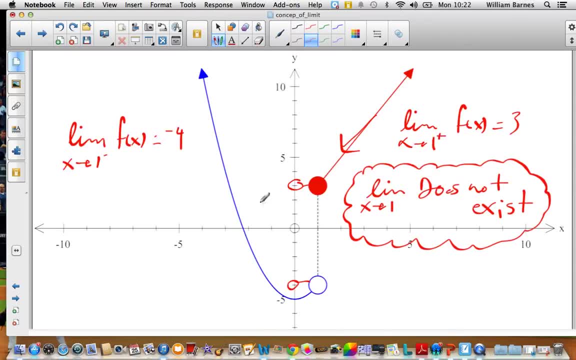 And tell: well, this one doesn't have a jump, This one has a jump. discontinuity here, All right. So let's look at one last example That you might see in calculus class, And these are the kind of monotonous examples. 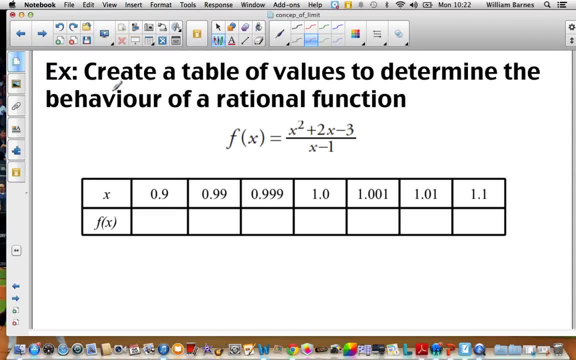 But anyway, So you have a function And your professor asks you to- Or your teacher Me Asks you to- Evaluate the one side limits By making a chart. So it's kind of the same thing Numerically As it was visually. 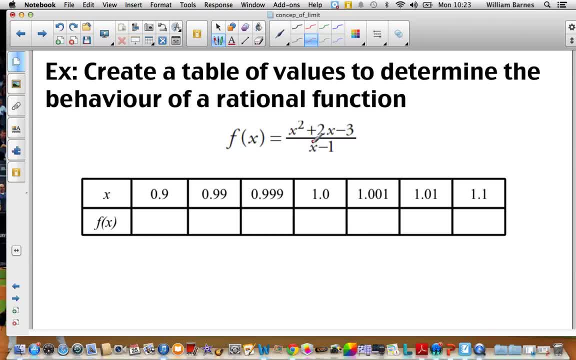 But you notice right away Is that I have Division by zero, So I have a non permissible value At x equals one, Or discontinuity, Point of discontinuity, Whatever you want to call it. So right here I have no idea what's happening. 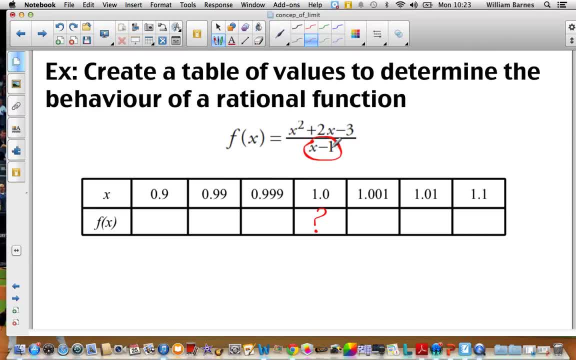 That's the hole in our graph. That's all. it is The hole in our graph. So if I, you know, subbed in 0.9.. Into this guy. You know This factors to X minus one, X plus three. 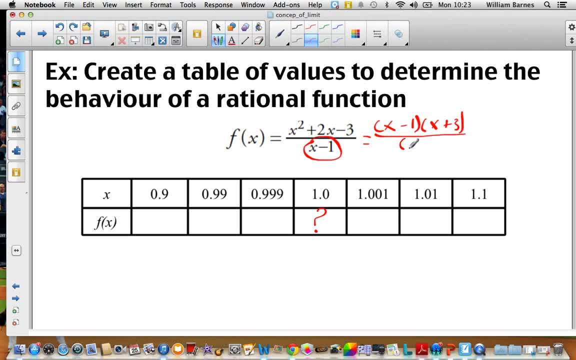 All over X minus one, And what happens is this: cancels, And when you get cancellation like that, That means you have a point of discontinuity. So it will look like the first graph that we had, The parabola with the hole in it. 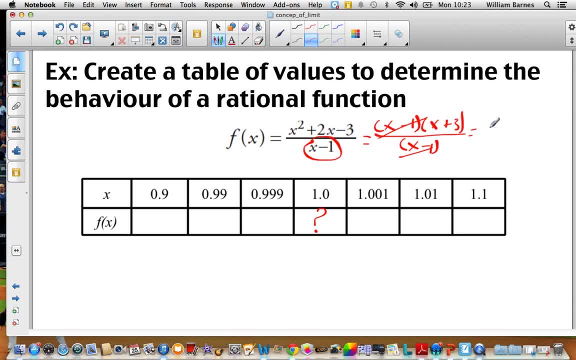 Essentially. Well, this one will actually be just a line with the hole in it, Because we're left with x plus three. So If I sub 0.9 into here, I'm going to have 3.9.. If I sub in 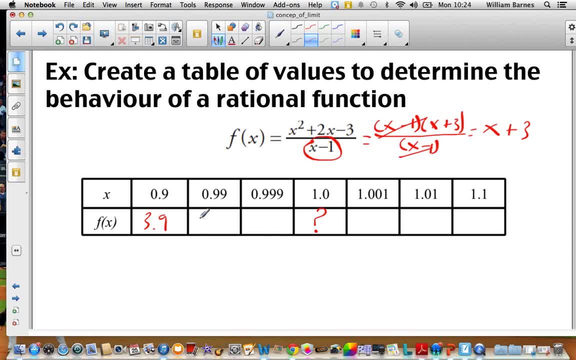 0.99.. You know I have 3.99.. I do the same thing here: 3.999.. So if you look at it, As I'm approaching One From the left side, So From the left side. 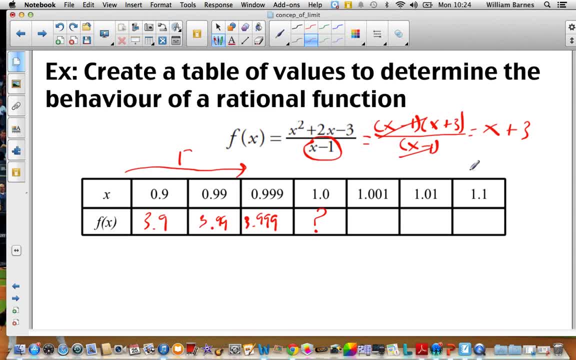 It looks like I'm approaching four And I'll do it over here, From the, From the right side. So it's going to be 4.001.. 4.01.. 4.1.. So if I come from the right side, 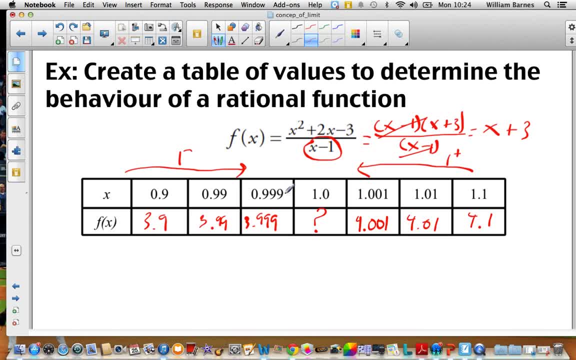 Again, I'm getting closer and closer to four. I could keep making this 4.99999999. And I still. Each time I keep getting closer and closer to four. So what I can say In this situation Is: x approaches four. 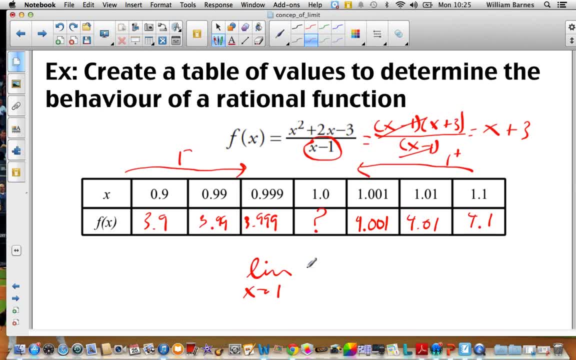 Or, sorry, one Of this f of x. I'm not going to write it out. You should. if you're on a test, You should write the whole thing out: Is four, Because both one sided limits are approaching the same number. So, guys, I hope this helps. 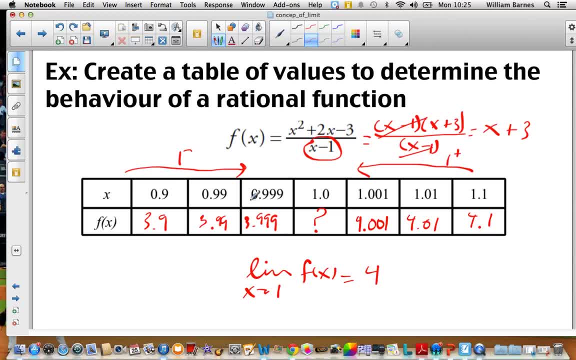 If you're looking for some more concrete examples Of how to do limits, Indeterminate values, Things like that, You should go check my page. I got a ton of videos on This stuff. on a test, You're going to be asked how to use this stuff. 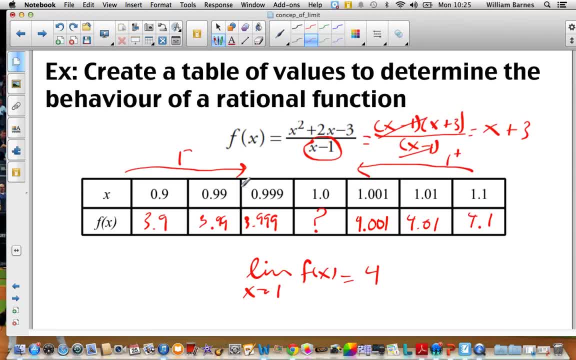 But it's still fundamental to understanding calculus, Which is really important, And how to pass calculus. You have to really think about it on a much deeper level And do lots of questions, So Hope this helps.